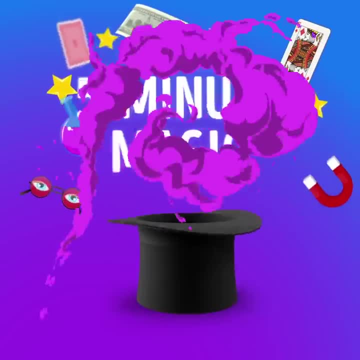 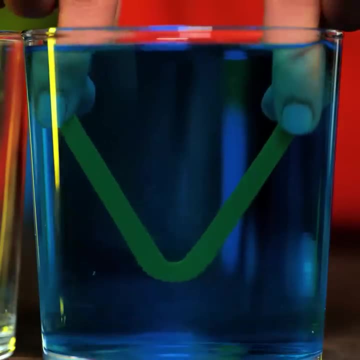 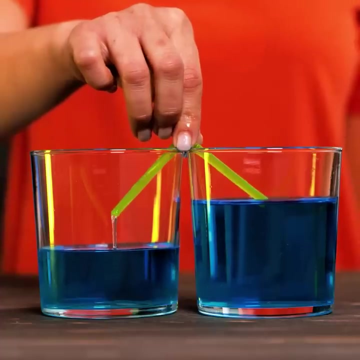 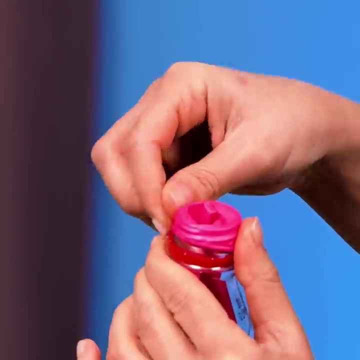 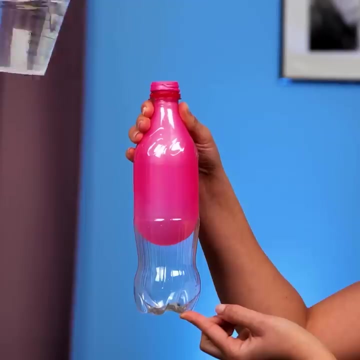 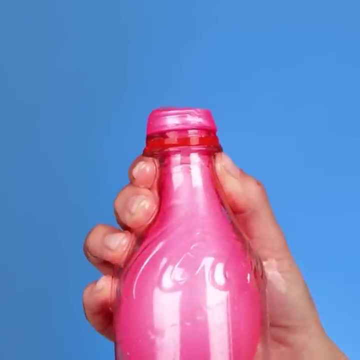 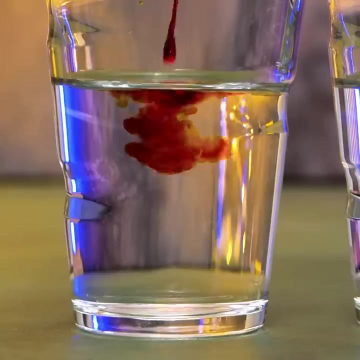 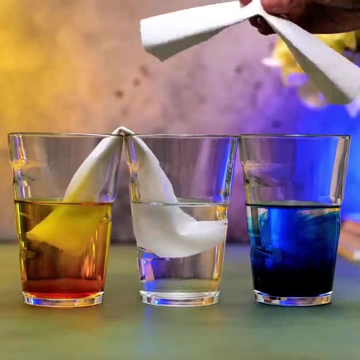 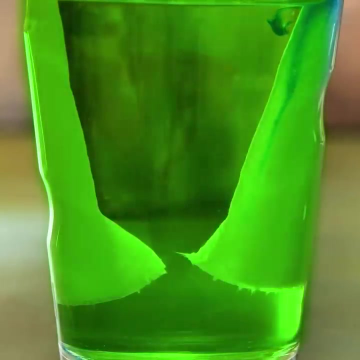 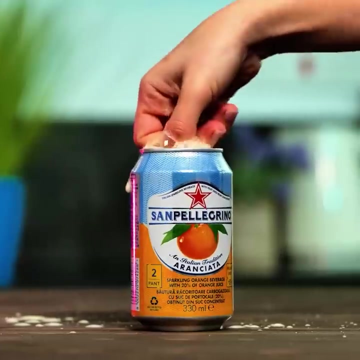 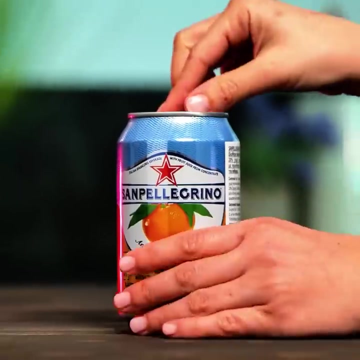 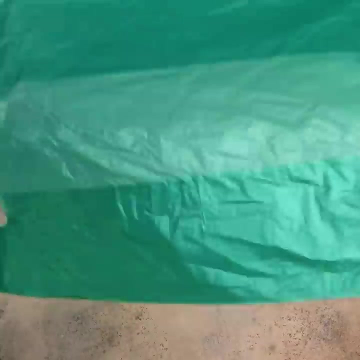 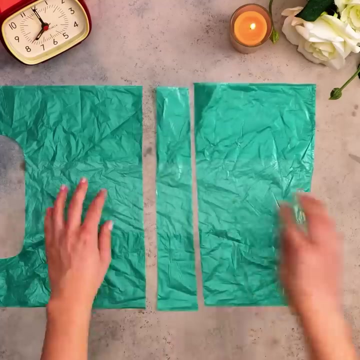 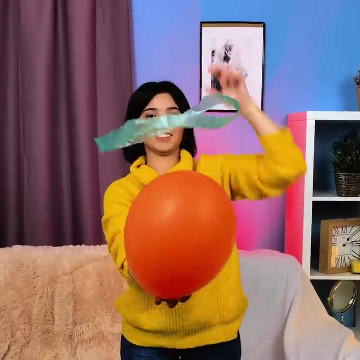 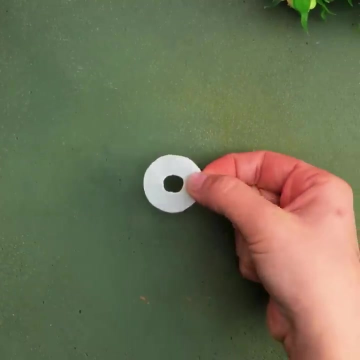 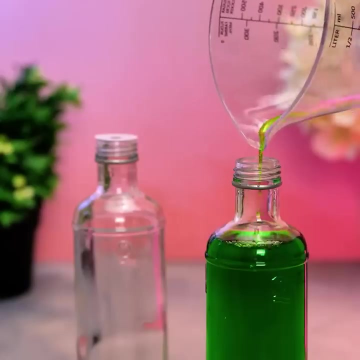 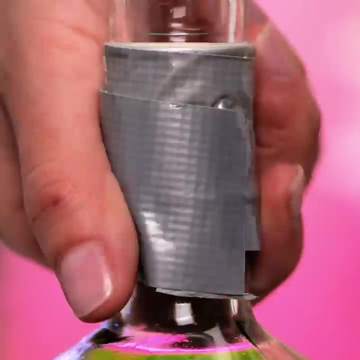 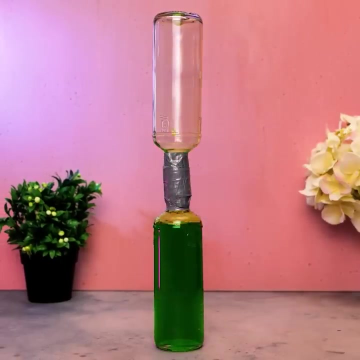 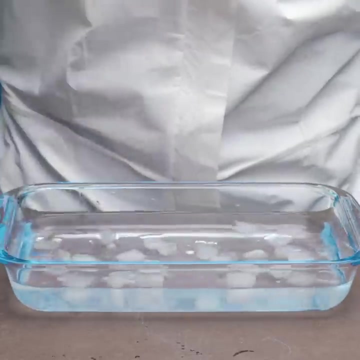 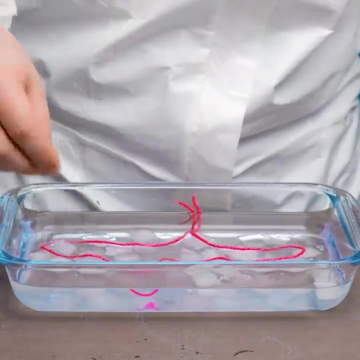 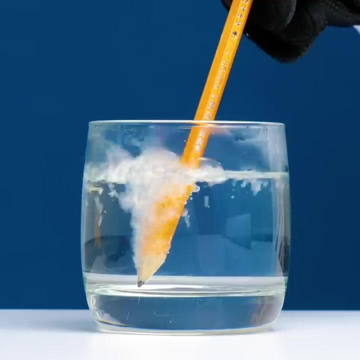 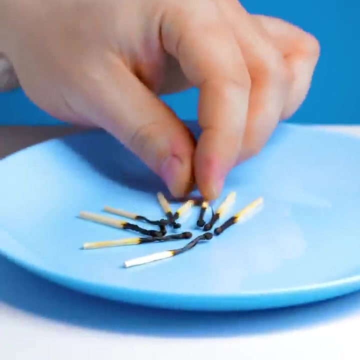 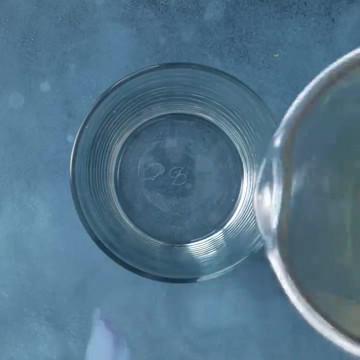 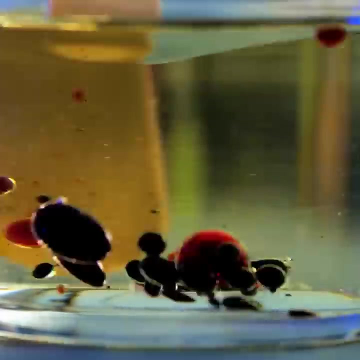 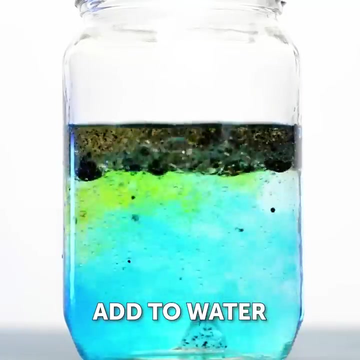 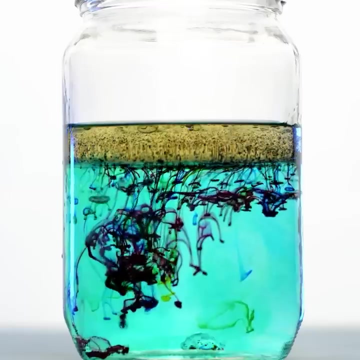 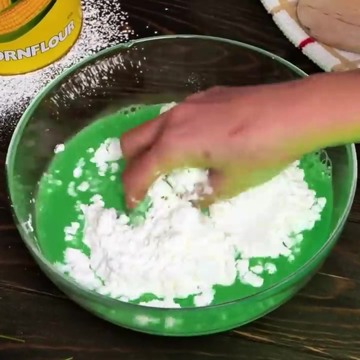 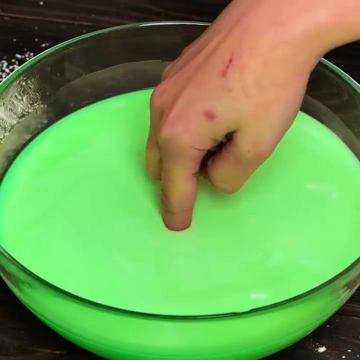 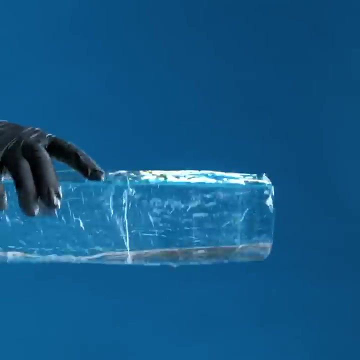 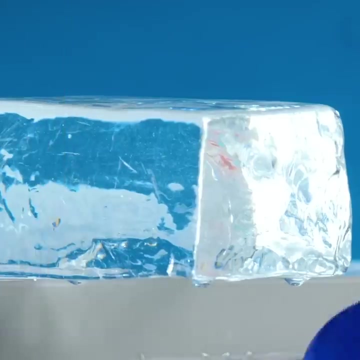 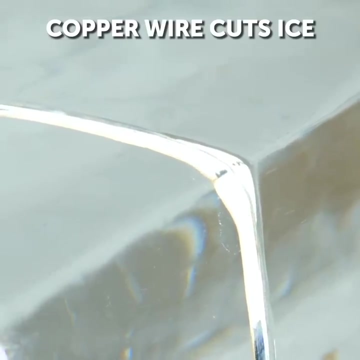 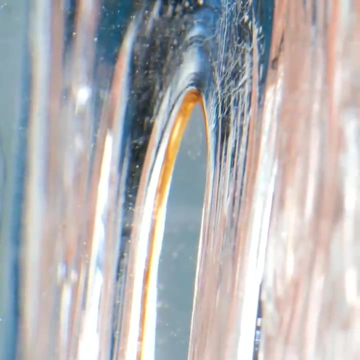 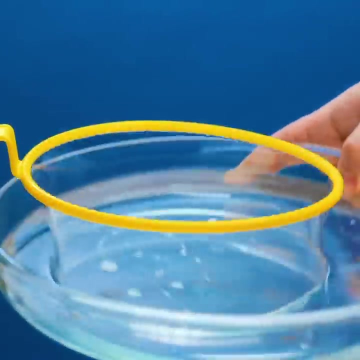 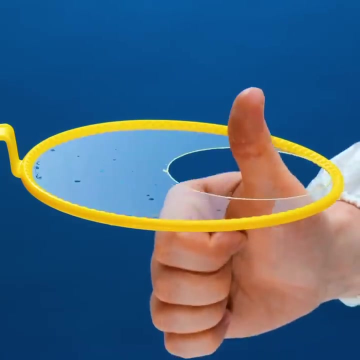 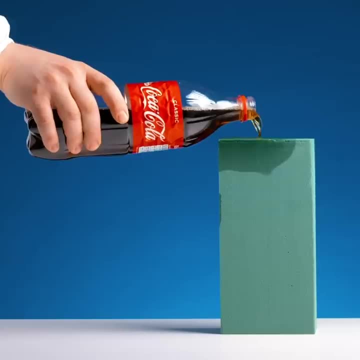 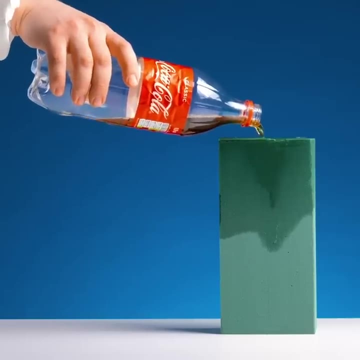 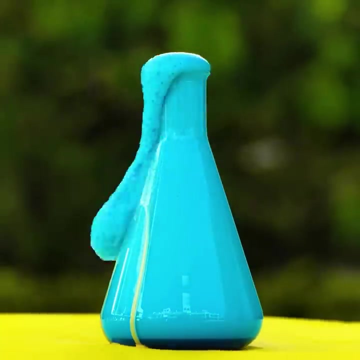 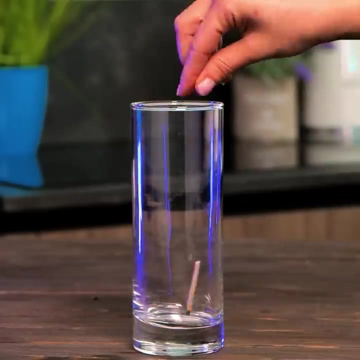 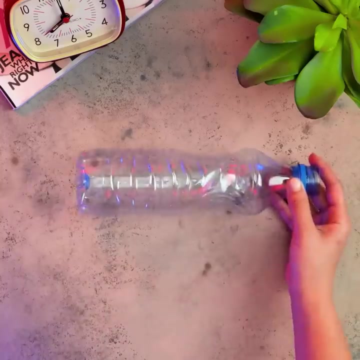 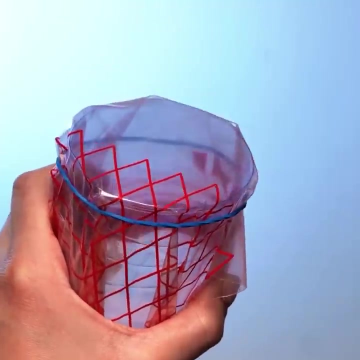 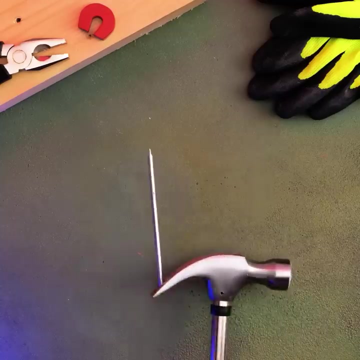 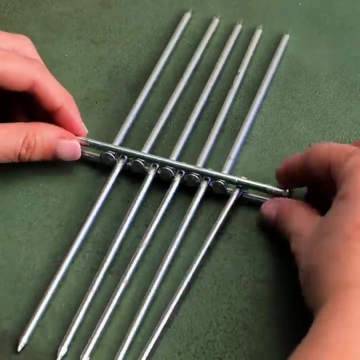 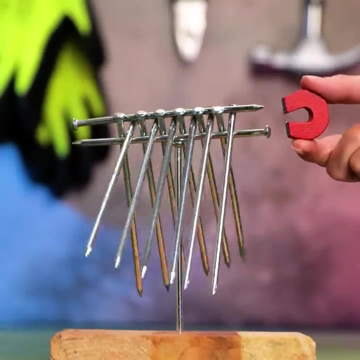 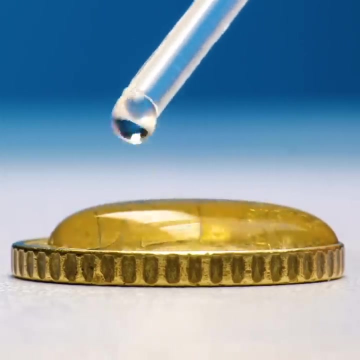 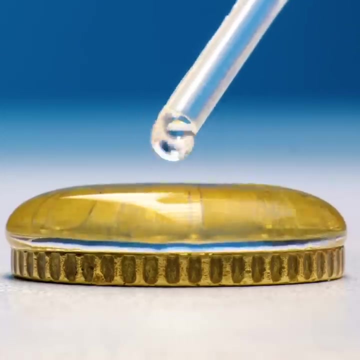 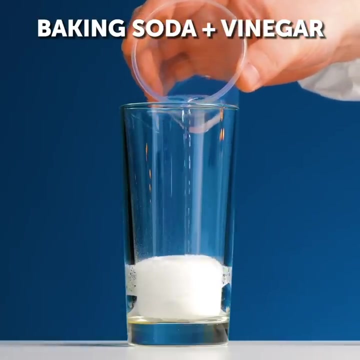 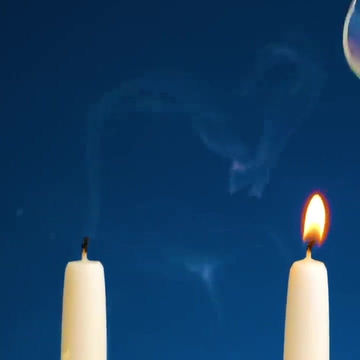 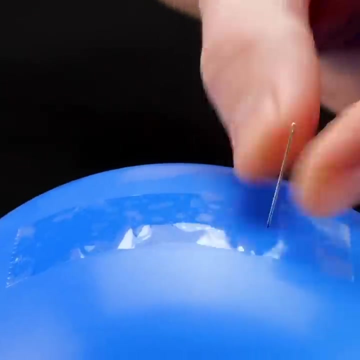 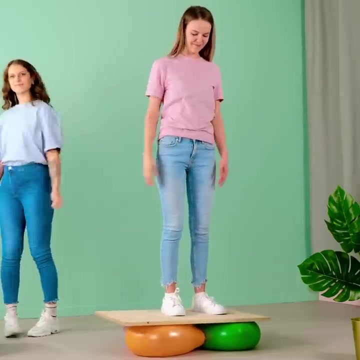 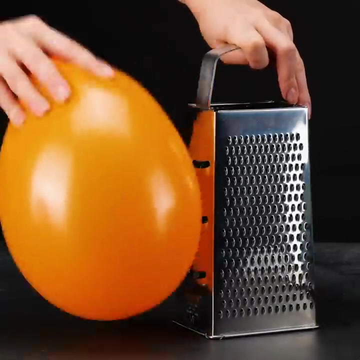 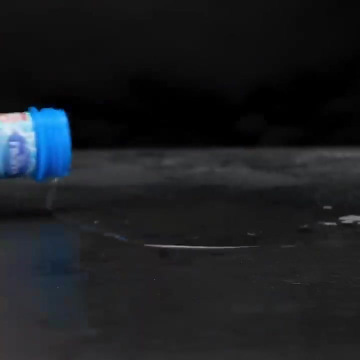 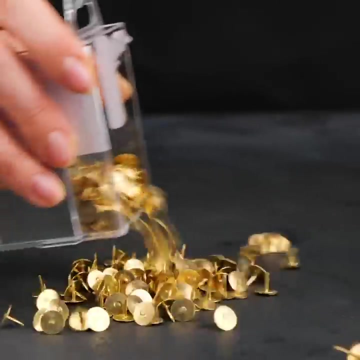 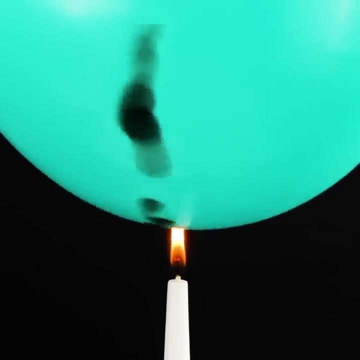 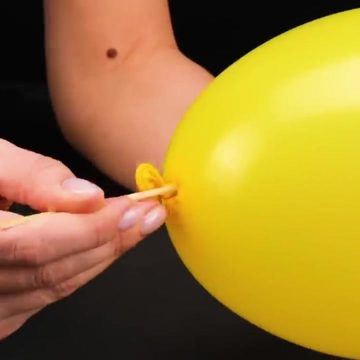 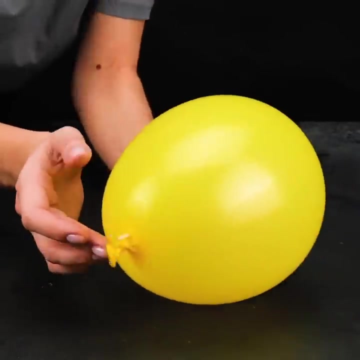 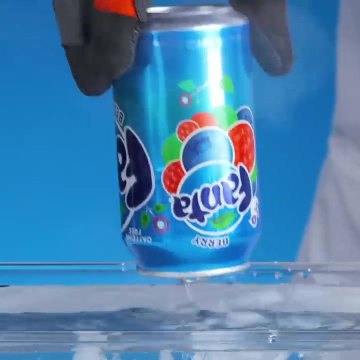 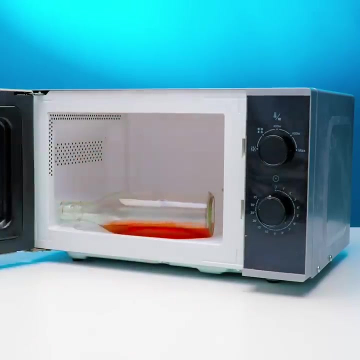 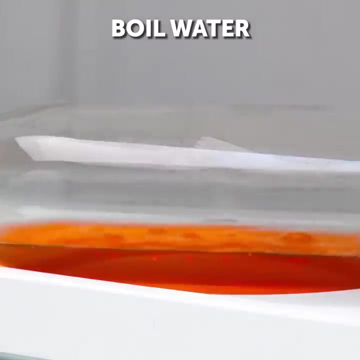 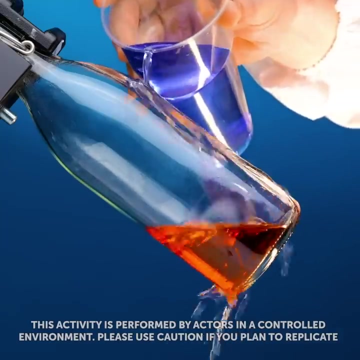 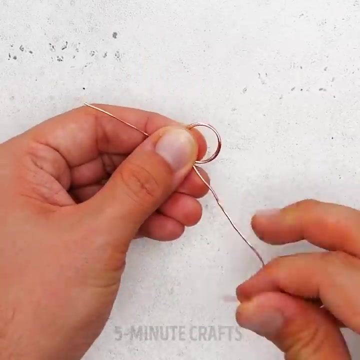 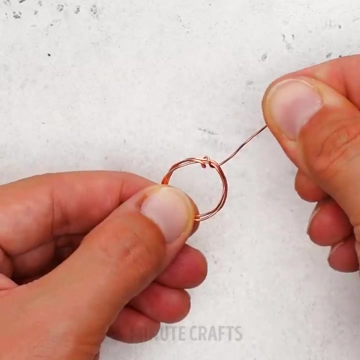 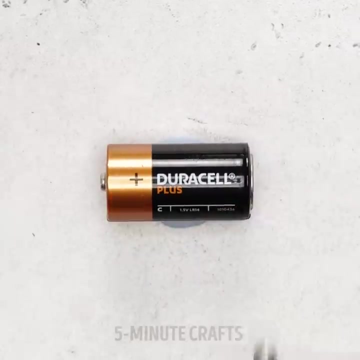 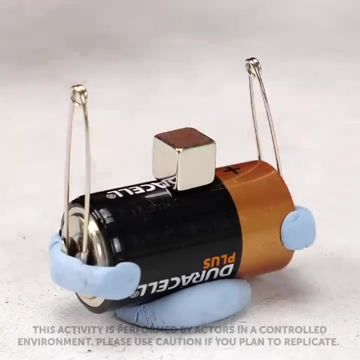 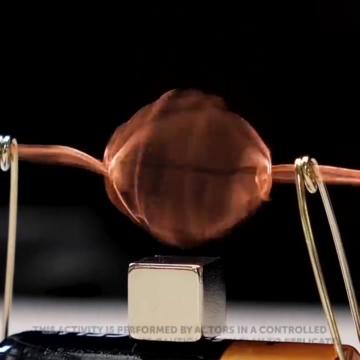 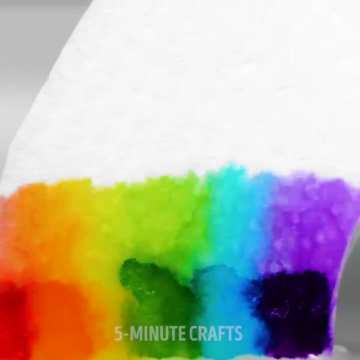 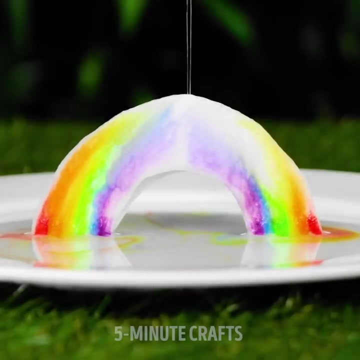 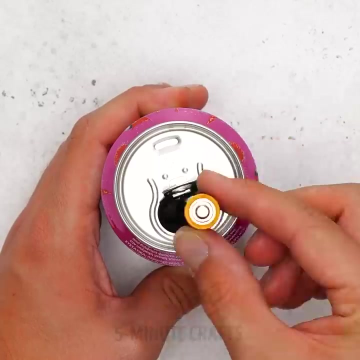 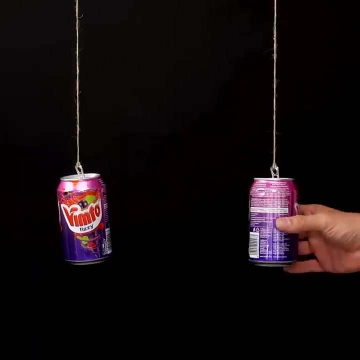 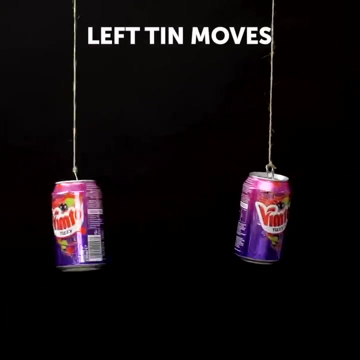 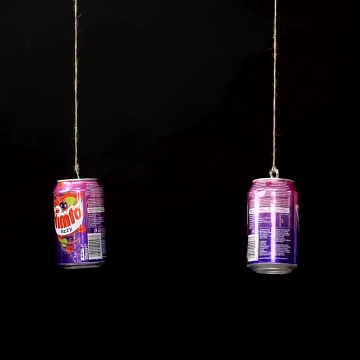 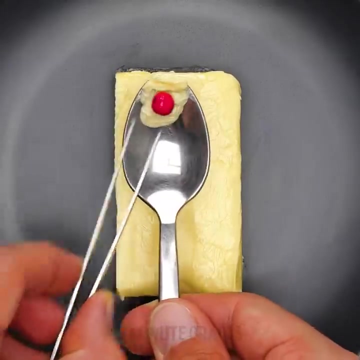 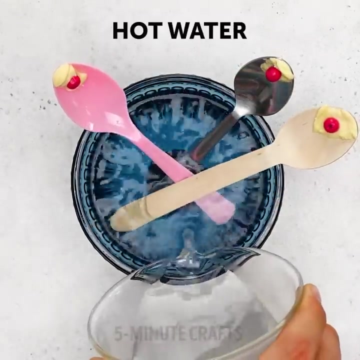 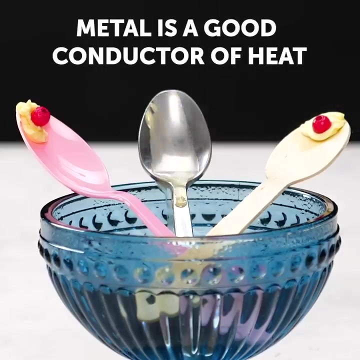 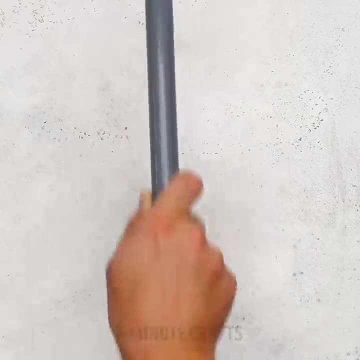 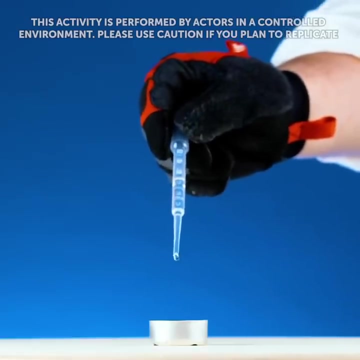 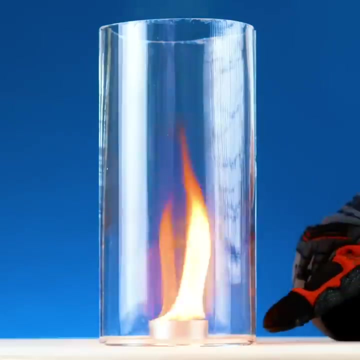 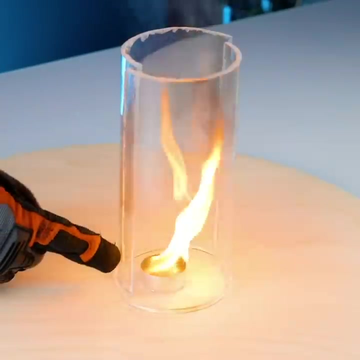 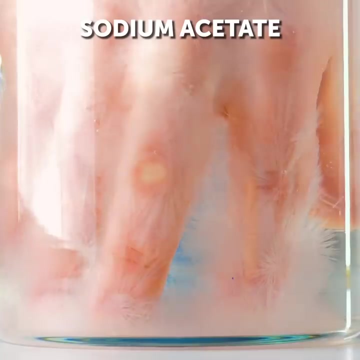 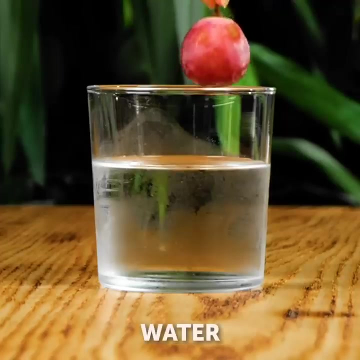 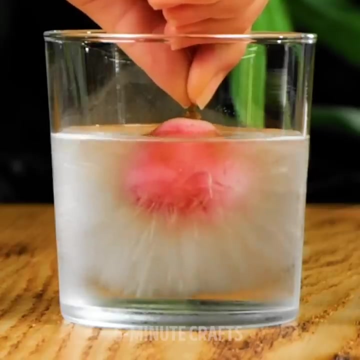 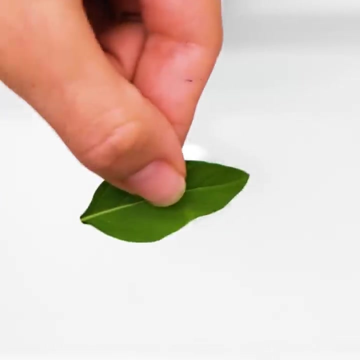 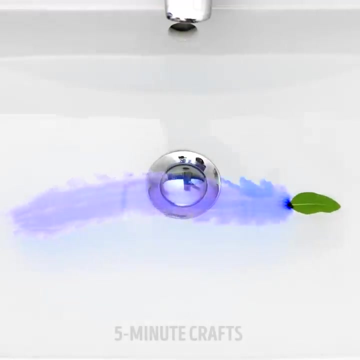 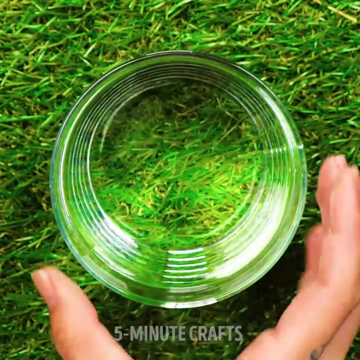 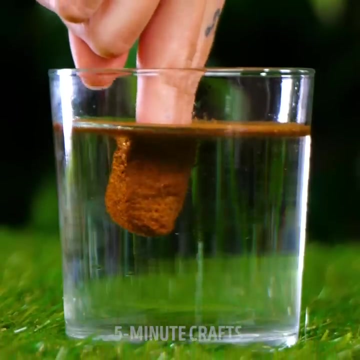 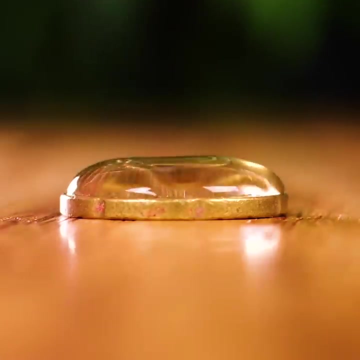 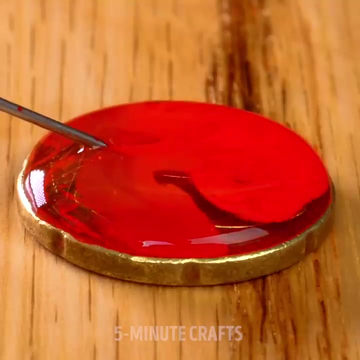 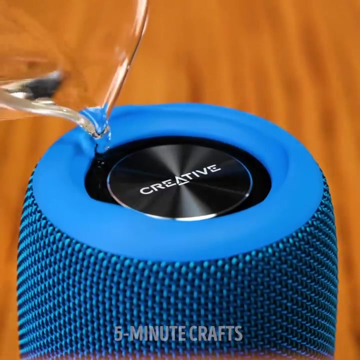 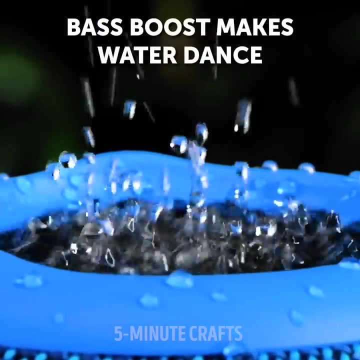 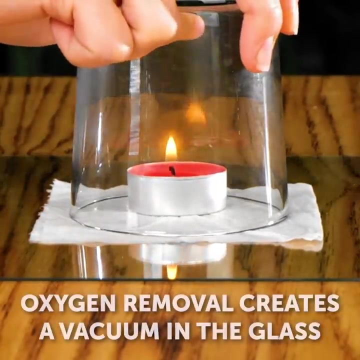 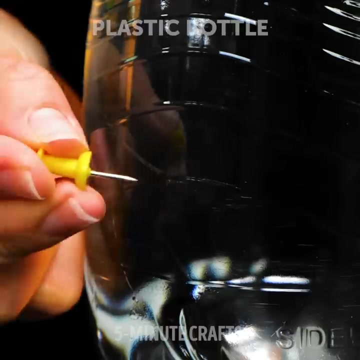 Thank you for watching. Thank you for watching, Thank you for watching. I just can't be without you, baby, Want you all night long. Want you all night long. Want you all night. want you all night. Tell me Why'd you have to go and drive me so crazy? 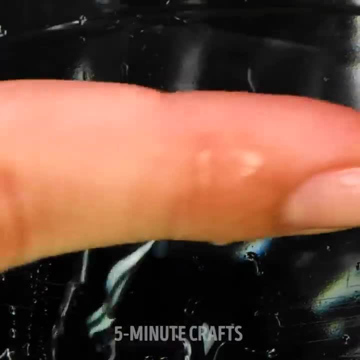 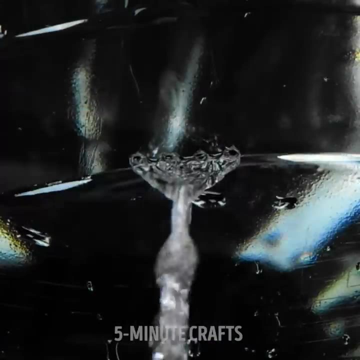 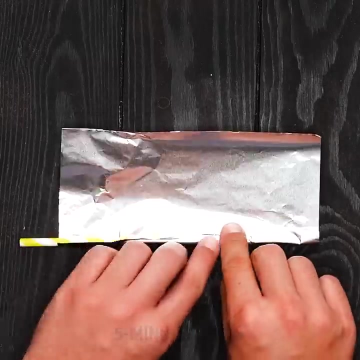 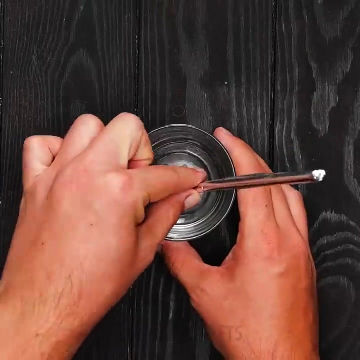 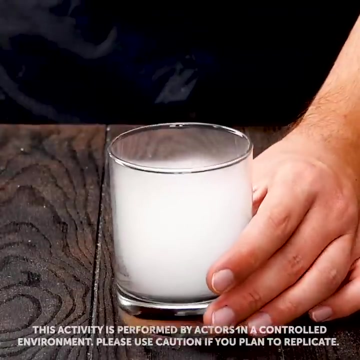 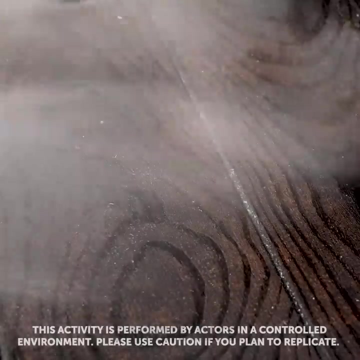 Now I'm feeling lost without you and I just can't be Without you. baby Want you all night long. Want you all night long. Tell me, Baby, Now I'm feeling lost without you and I just can't be Without you. baby Want you all night long. 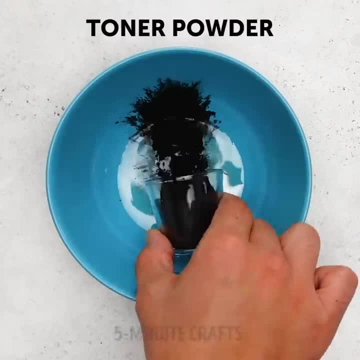 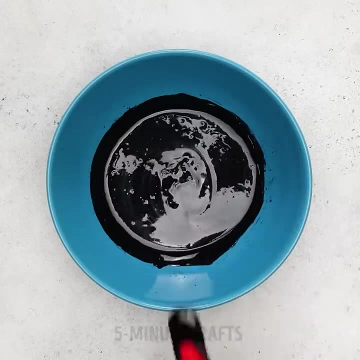 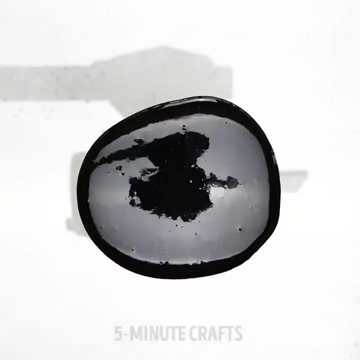 Want you all night long. Give me all your love. Baby, give me all your love. Baby, give me all your love, All your love, all your love. Give me all your love. Baby, give me all your love. Baby, give me all your love, All your love. 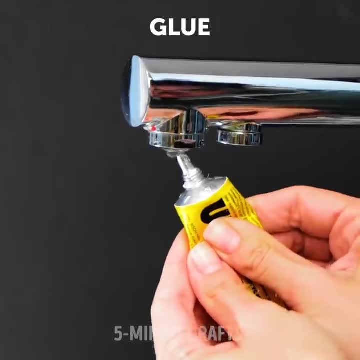 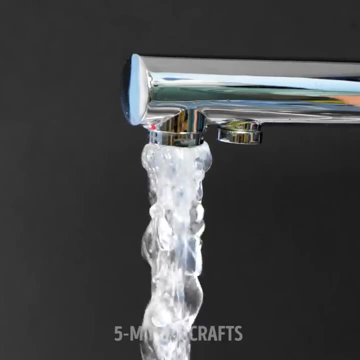 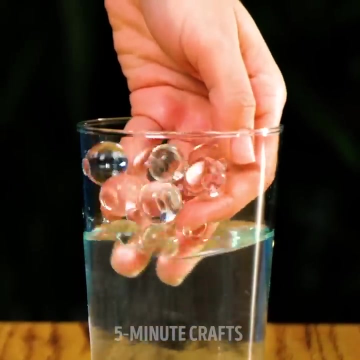 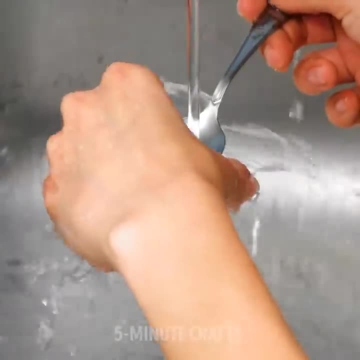 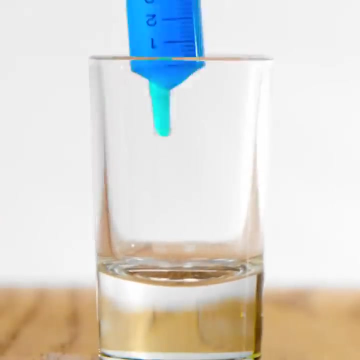 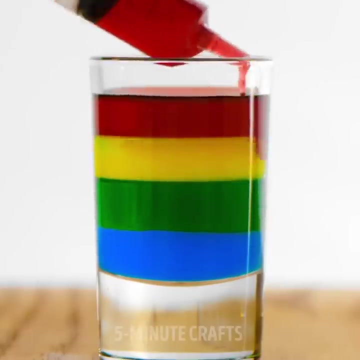 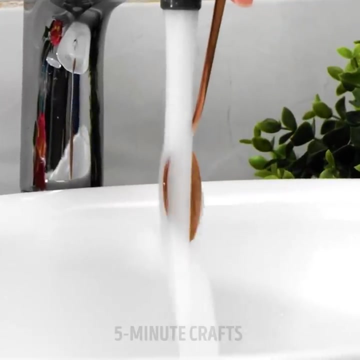 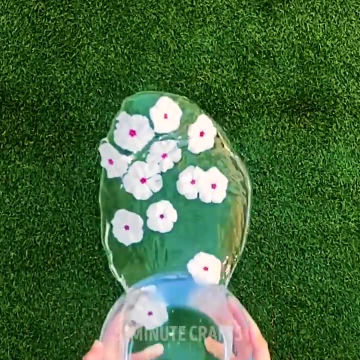 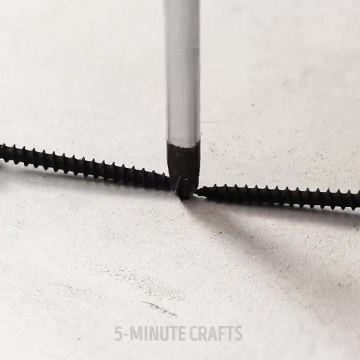 Without you. baby, Want you all night long. Want you all night long. Get up, get up, do it. Don't wait. We're talking to each other. I know we feel the same About the situation, Like we're stuck inside a game Time to get out of this circle. 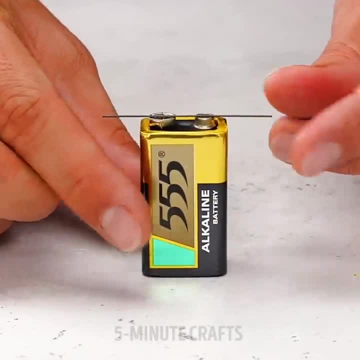 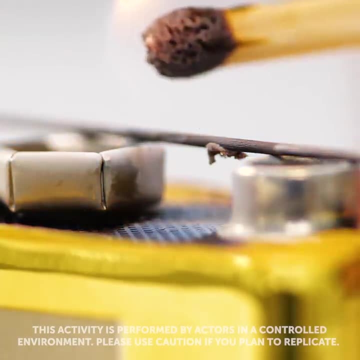 Yeah, we both carry a scar As you write the part we're playing. Time to cherish who we are, Time to cherish who we are. The only thing I ever wanted Starts with us taking the chance. Starts with us taking the chance, Not like anything we've done before. 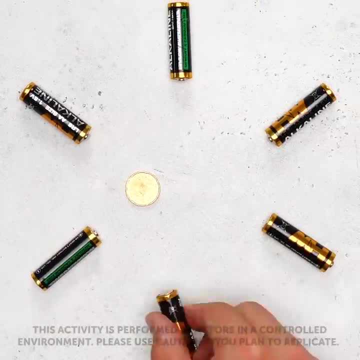 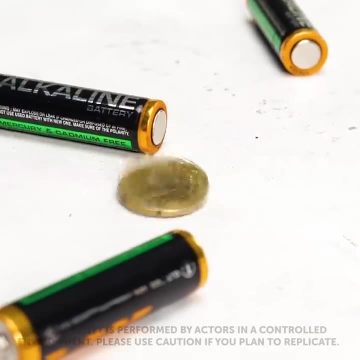 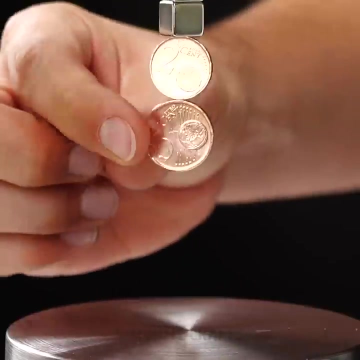 Not like anything we've done before. Yeah, Now it's time for something better And time for us to follow our dreams. No, we can't stay, no more. Come, run away. Don't be afraid, We'll be okay And I know it's the right thing to do. 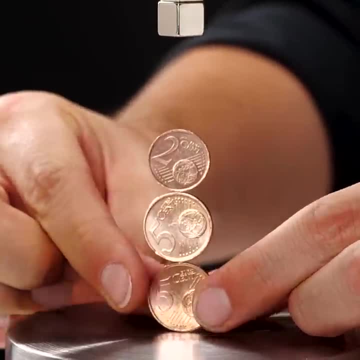 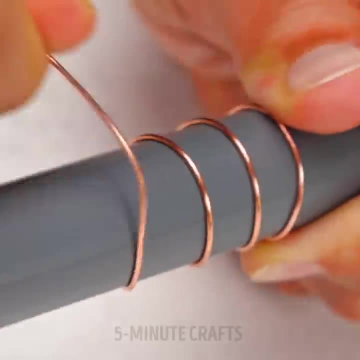 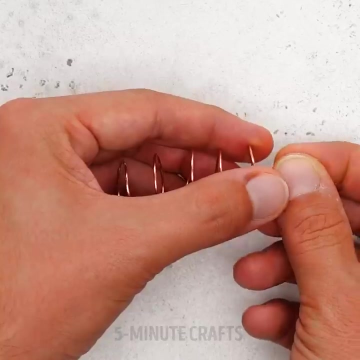 Let's break away, All colors will fade. Let's go our own way. There's no time to decide what to do. And I'll say There's no time to decide what to do, And I'll stand by you, By you, And I'll stand by you, And I'll stand by you. 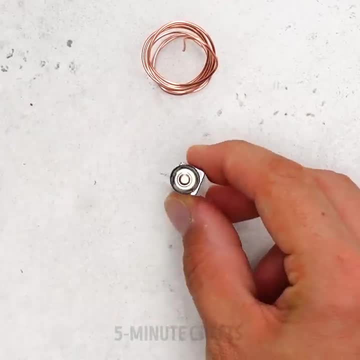 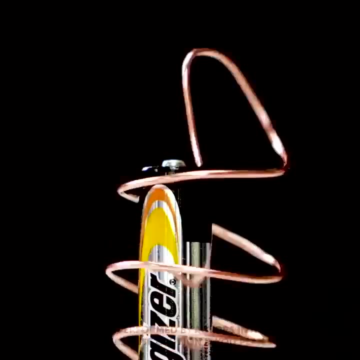 There's no time to decide what to do. Let's break away, Get up, get out. do it break away. get up, get out. do it break away. Get up, get out, do it break away. It's always mixed emotions.